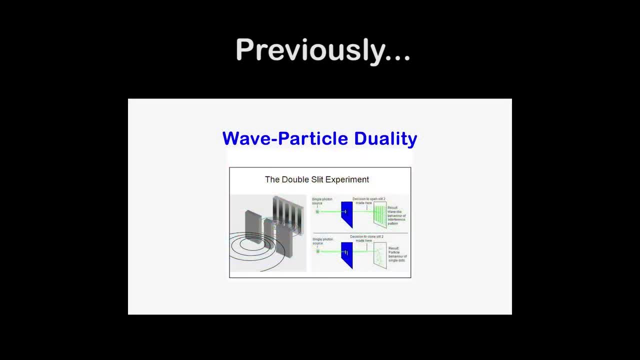 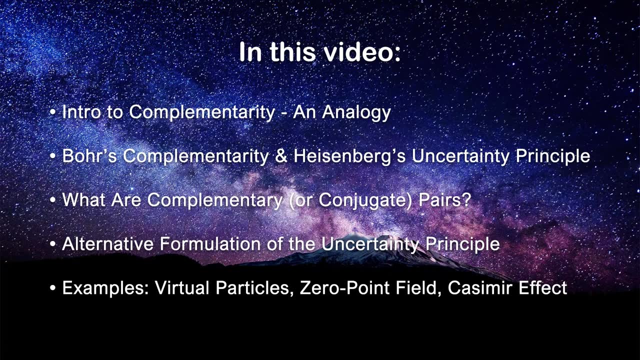 the uncertainty principle are intimately related. I also mentioned that wave-particle duality is a type of complementarity. Well, in this video I'll dig a little bit deeper by exploring how Heisenberg's uncertainty principle and Bohr's complementarity arise together in quantum. 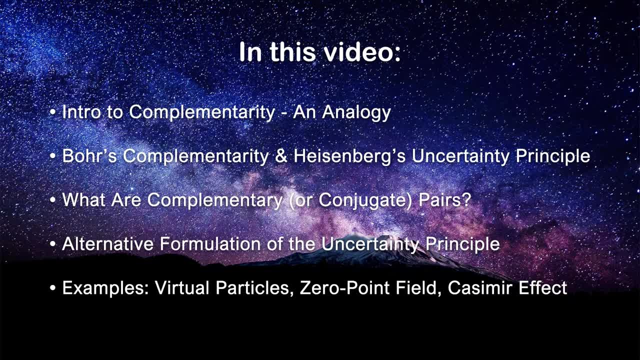 mechanics. In addition, in the second part of the video, I'll cover an alternative form of the uncertainty principle and I'll illustrate its significance by using a fascinating example. I'll explain how this other form of the uncertainty principle explains the existence of virtual 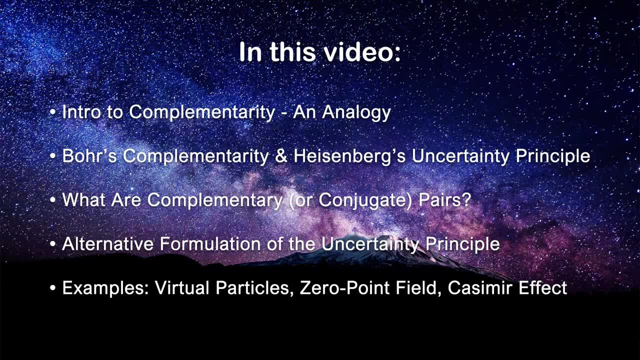 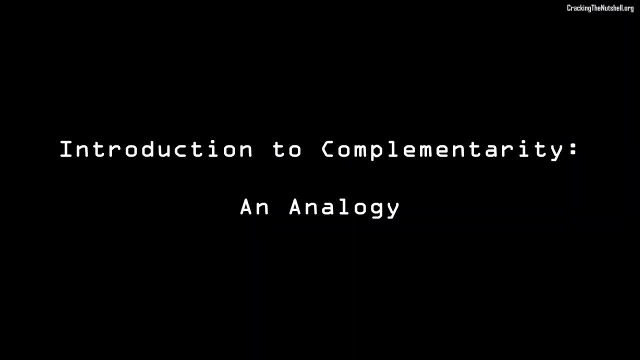 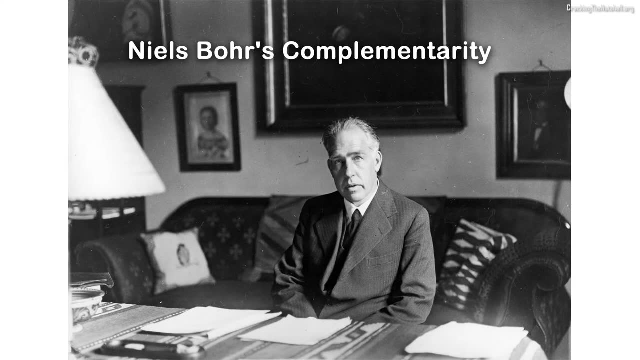 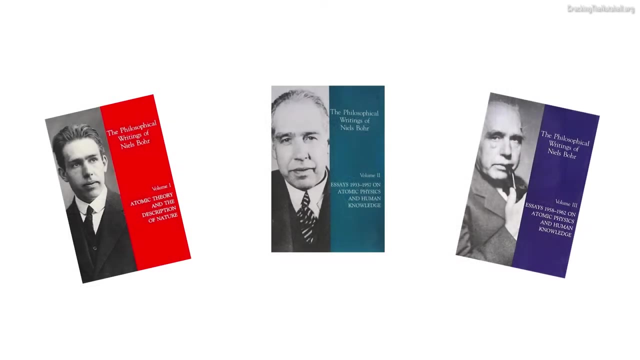 particles, the zero-point field and the Casimir effect. Let's get started. Complementarity is a concept which was introduced by physicist Niels Bohr, one of the founding fathers of quantum theory, at the beginning of last century, Even though Bohr himself never actually gave an explicit definition of what he meant by. 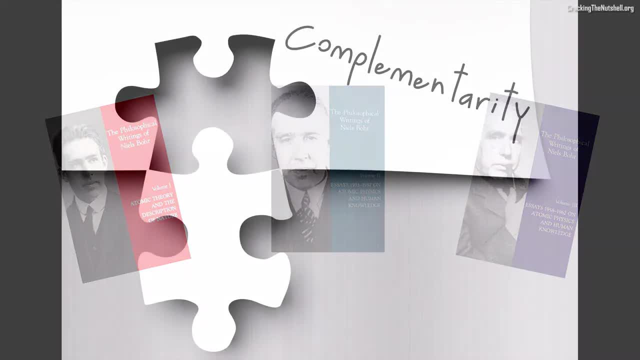 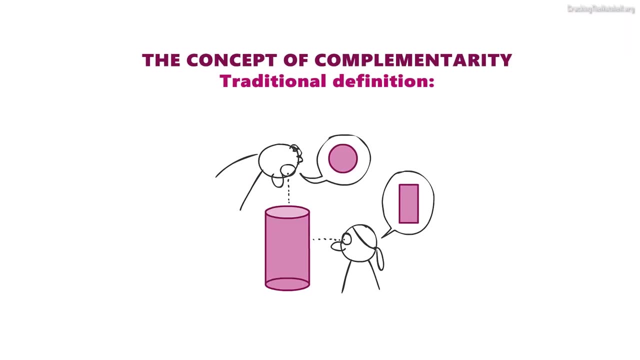 complementarity. what we do know is that the term, whenever it appears in his writings, is not to be taken in its usual sense. Let me explain. Usually, when we talk about two complementary descriptions of the same object, we mean that while these descriptions are partial, they are not in any way opposed to. 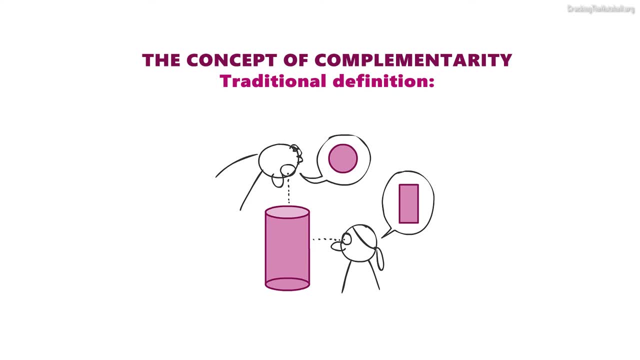 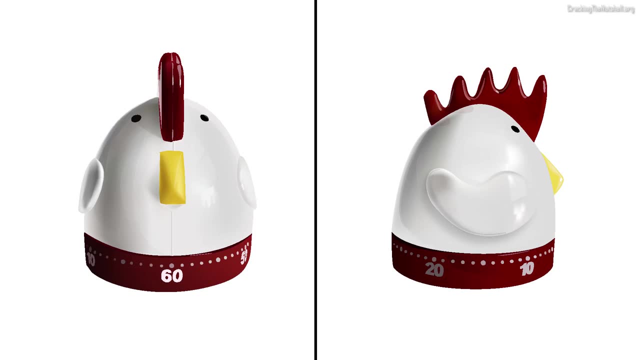 one another. We say that they are complementary to each other. Let's use an analogy to illustrate what I mean. Imagine we take two different photographs of the same object, say one full face and the other one in profile. In the ordinary sense of the word, we can say that these two photographs are complementary. 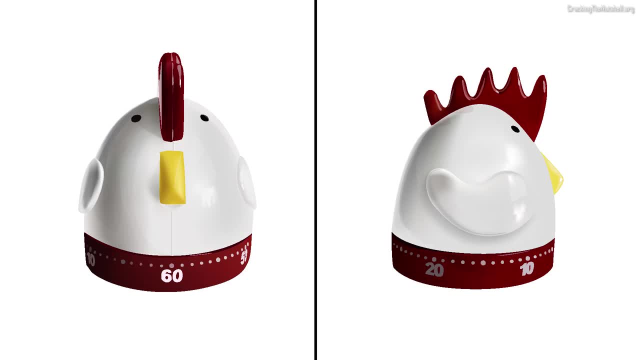 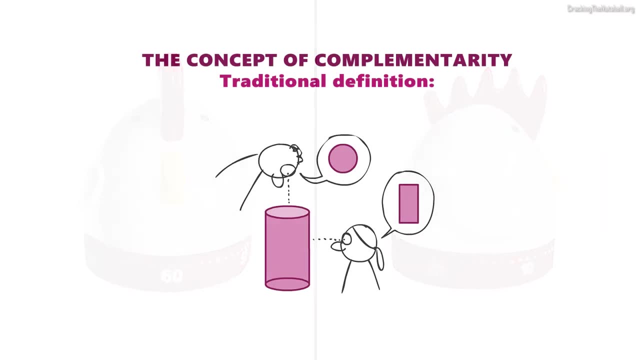 to each other, since when they are combined, they yield a more detailed knowledge of the object in question as it existed in that particular moment in time. However, this idea of complementarity is not what Bohr had in mind. According to Bohr, 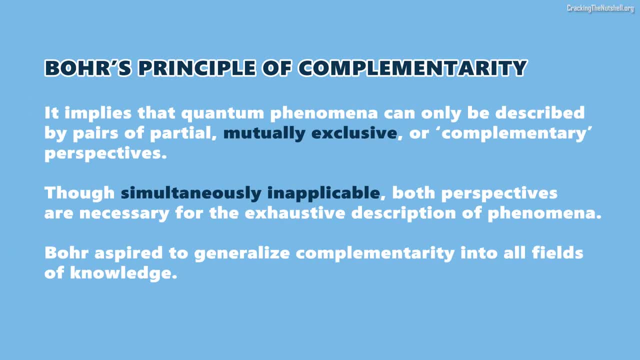 when it comes to quantum entities, the act of combining any two pictures of the same object at any particular moment in time in order to form a more detailed description of certain pairs of properties is actually impossible. This is because, when it comes to the quantum world, it is in fact not possible. 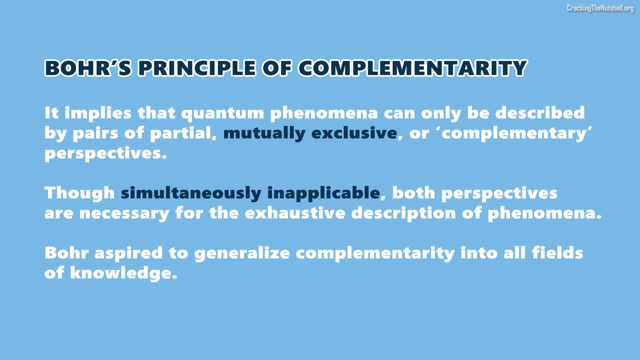 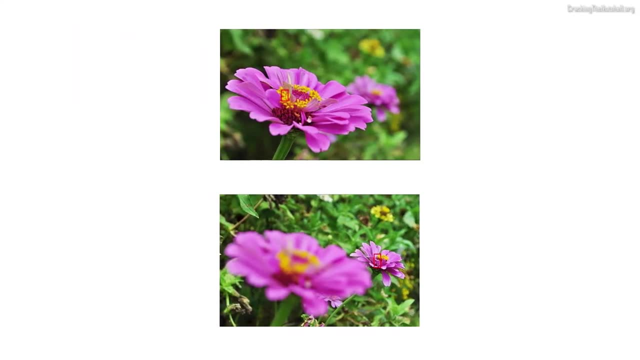 to perform simultaneous joint measurements of the physical quantities corresponding to certain pairs of properties. Continuing with the photoanalogy, we could argue that Bohr's notion of complementarity can perhaps be better understood when we look at the situation when we aim to take a picture. 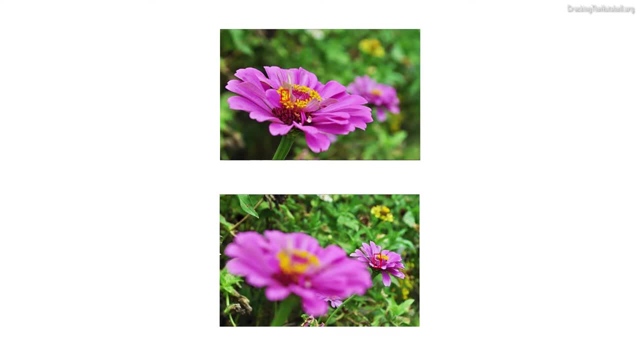 of a landscape showing several planes using a wide-angle camera. Whenever we focus on the foreground, the background appears fuzzy, and whenever we focus on the background, the foreground appears fuzzy too. There is a clear trade-off of information here. depending on how much focus we place on any particular plane, The more we know about the foreground. 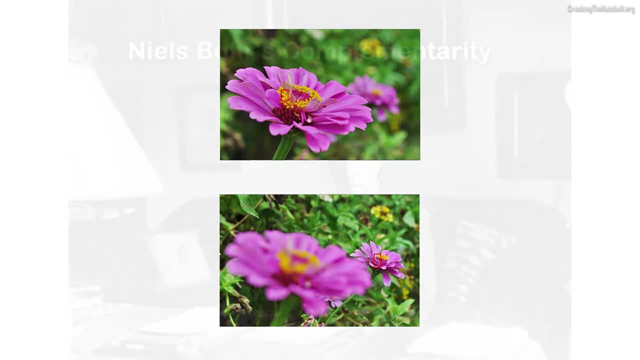 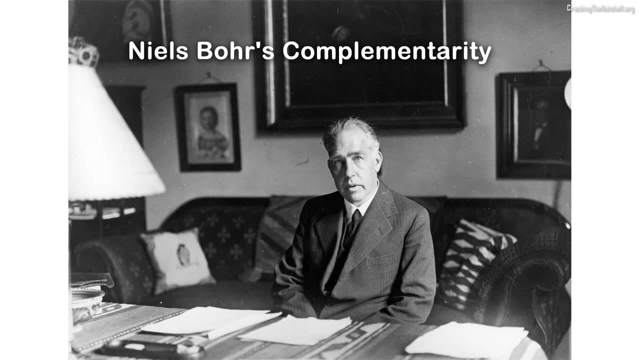 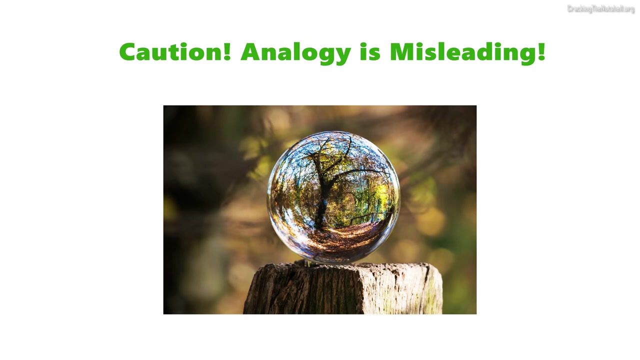 the less we know about the background, and vice versa. This analogy definitely gives us a better idea of what Bohr meant by complementarity. However, we must be cautious, because it is actually quite misleading. It implicitly assumes the simultaneous existence of all the objects and their properties lying in 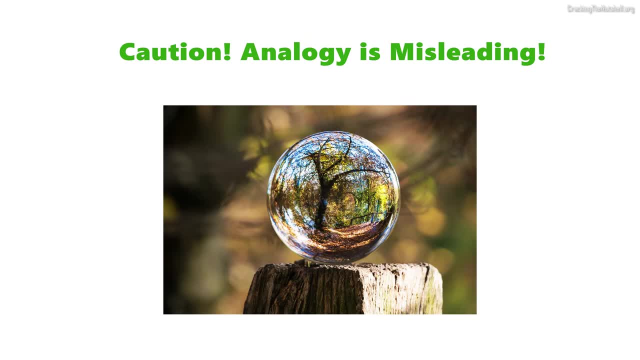 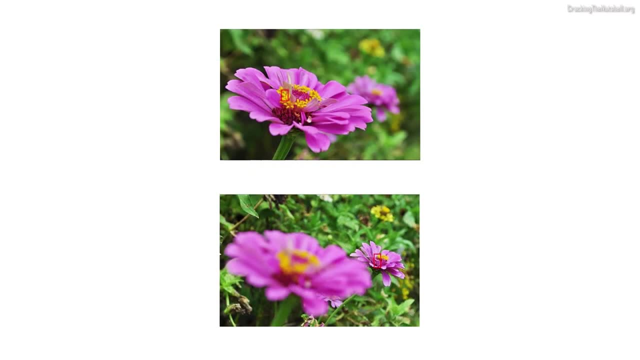 the different planes. It assumes an existence independent of the photographer's choices and his instruments of measurement. in this case the camera In the quantum world. background and foreground cannot be simultaneously defined in and of themselves. In other words, in Bohr's. 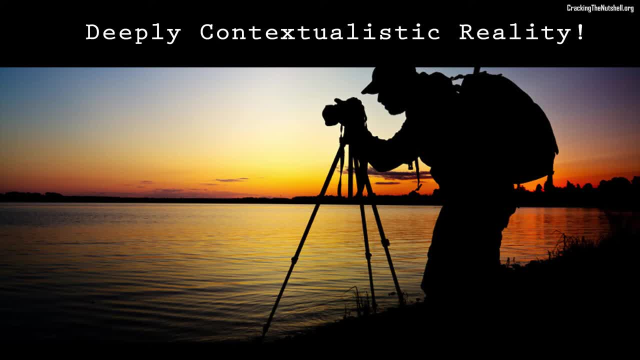 view, the manifestation of the properties in quantum photography can be almost completely supply and demand of a simple study as a conventional perspective. Enough is enough. This is an estabanpultein of authors é question, and hence the objects themselves actually would depend on the experimental. 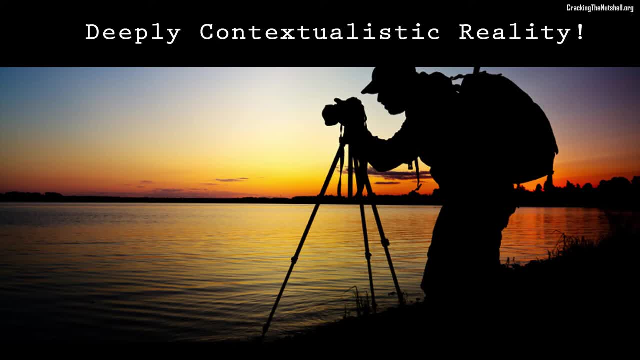 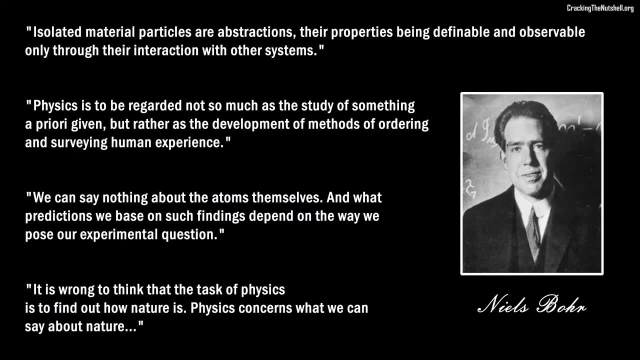 conditions, the instruments of observation and the photographer's choices. As I explained in my last video, Bohr actually denied that it is even meaningful to talk about the nature of a system per se, that is, to talk about its properties in themselves, independently of them being observed. Here we are talking not about a reality in itself. 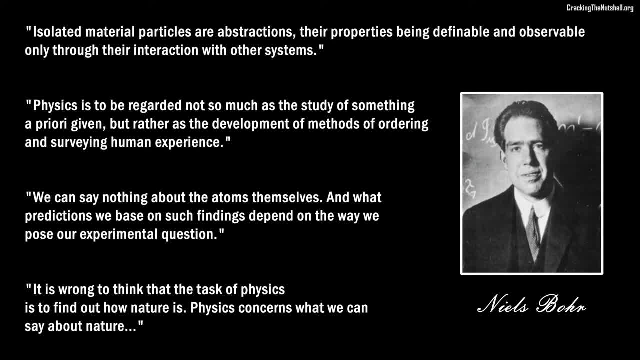 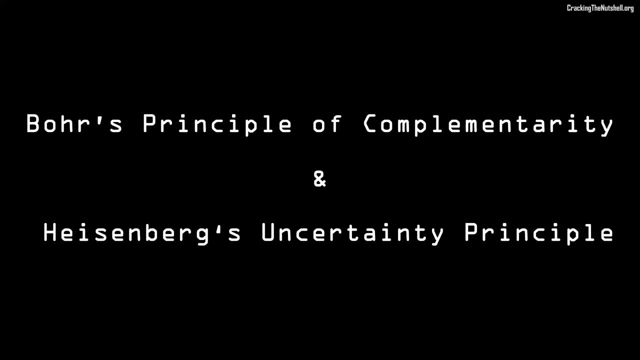 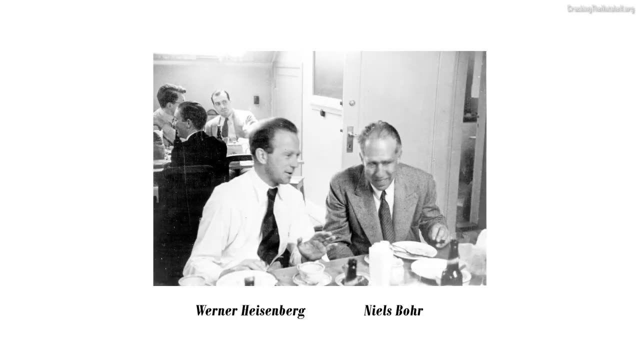 but about a deeply contextualistic reality. a reality which manifests differently in complementary ways, depending on the questions we ask. a reality which is inseparable from our instruments of observation and our modes of questioning. The principle of complementarity was formulated by Niels Bohr in 1927, shortly after receiving 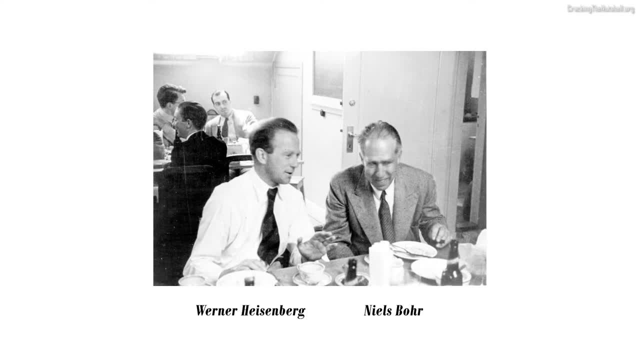 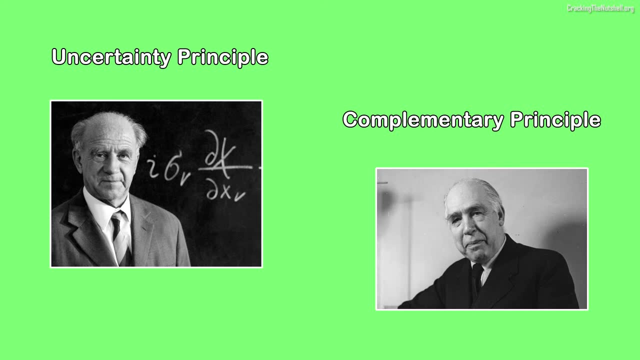 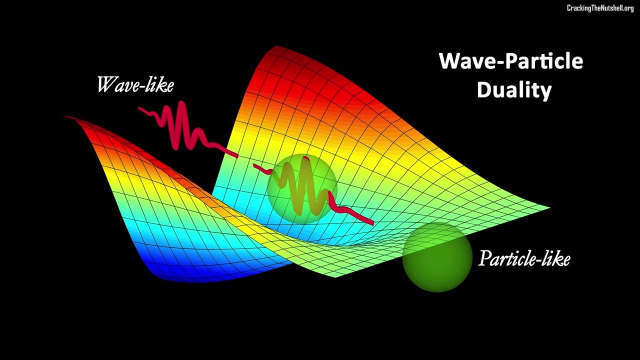 a letter from Werner Heisenberg regarding his newly-formulated theory of complementary uncertainty. Bohr saw Heisenberg's uncertainty principle as a particular mathematical formulation of a deeper concept of complementarity, and he argued that the proper derivation of the uncertainty principle should start from the indispensability of both particle and wave. 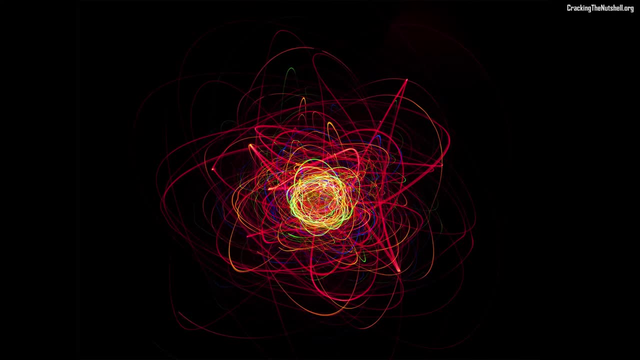 concepts. He pointed out that uncertainties in any experiment do not only arise from measurement disturbances, but that a deeper, more fundamental type of uncertainties arise from the fact that in any experiment, we need to take into account both the particle and the wave features. 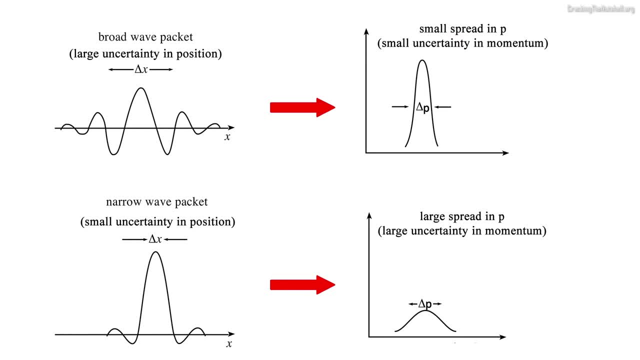 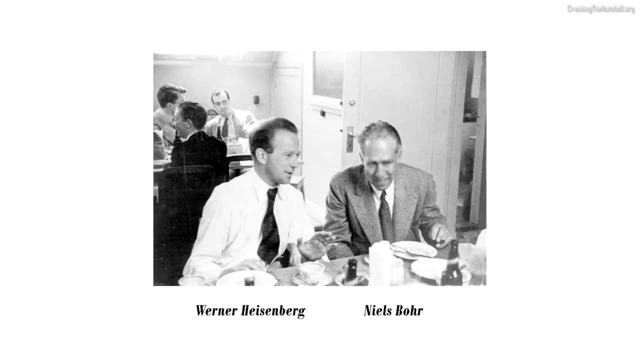 Throughout their exchanges, Bohr reminded Heisenberg that it is not so much the unknown measurement disturbance which renders the momentum of the particle uncertain, but rather it is the fact that the position and the momentum of the particle cannot be simultaneously defined. to start with, Bohr always stressed that the uncertainty relations are first and foremost 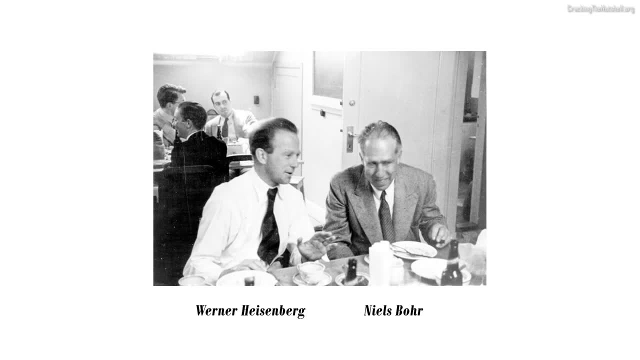 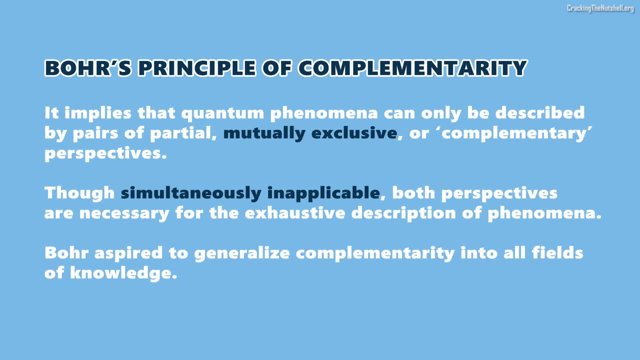 an expression of complementarity rather than a result of measurement disturbances. So what is the principle of complementarity then? The principle of complementarity holds that certain complementary phenomena cannot be made to simultaneously manifest fully. Wave-particle duality itself is an example of complementarity, for instance The choices 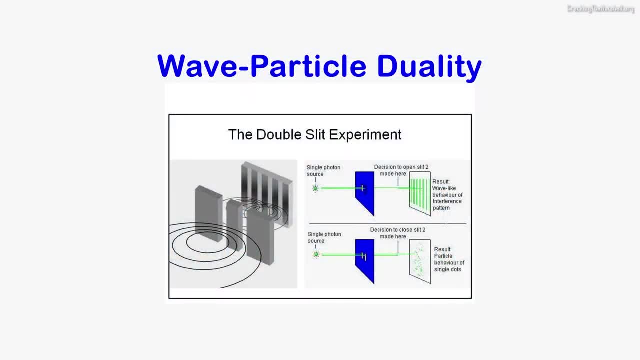 we make in our experimental setup will determine how particle-like or how wave-like our results will be. For instance, In the famous double-slit experiment, whether or not we decide to find out what slit the particle went through has a massive impact in the outcome of our experiment. If we look 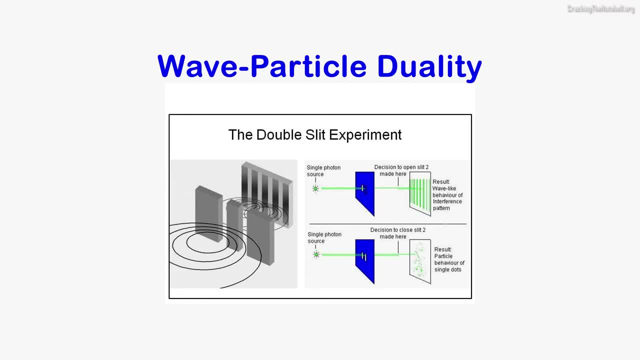 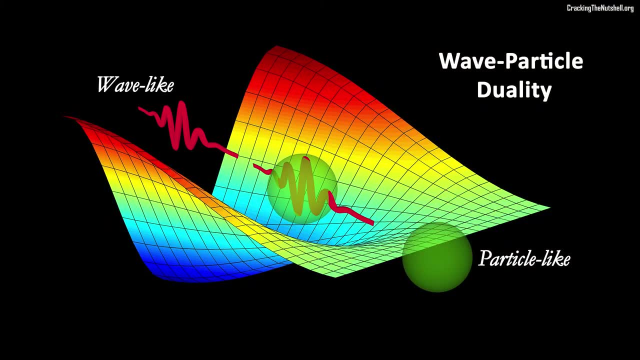 particle-like behaviour follows. If we don't look, a wave-like pattern appears on the screen. These wave-like properties and particle-like properties will manifest in such a way that there will always be a trade-off between them. In this way, it is impossible for us to measure. 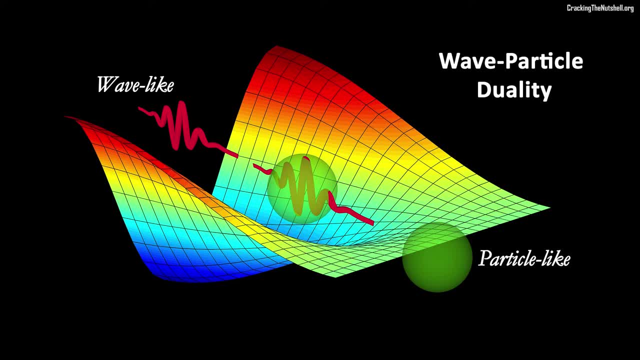 the four properties of a wave and the four properties of a particle In this way. it is impossible for us to measure the four properties of a wave and the four properties of a particle In this way. it is impossible for us to measure the four properties of a particle at any. 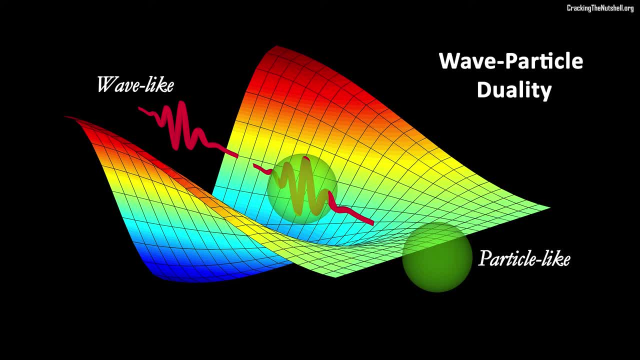 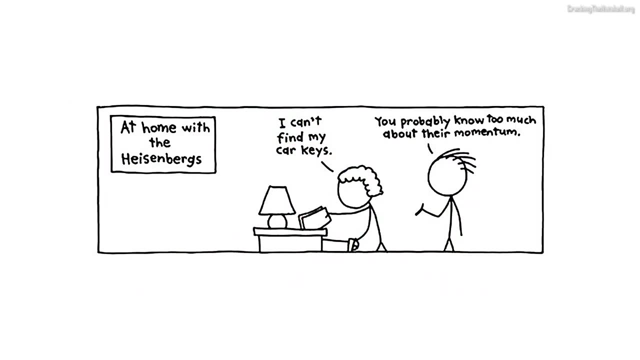 given moment. In fact, it can be argued that, in reality, there is no actual physical wave and that there is no physical particle either, As Bohr pointed out. all we can do is talk about properties that manifest through observation and about the way nature limits the simultaneous. 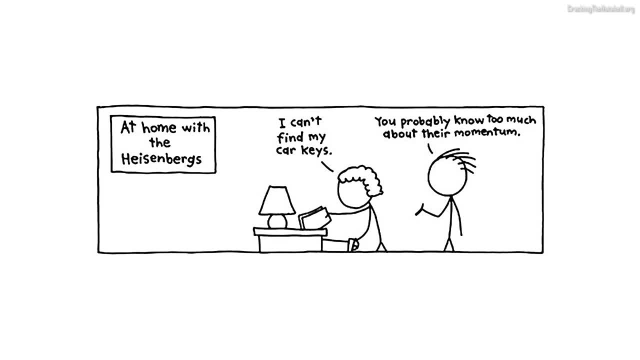 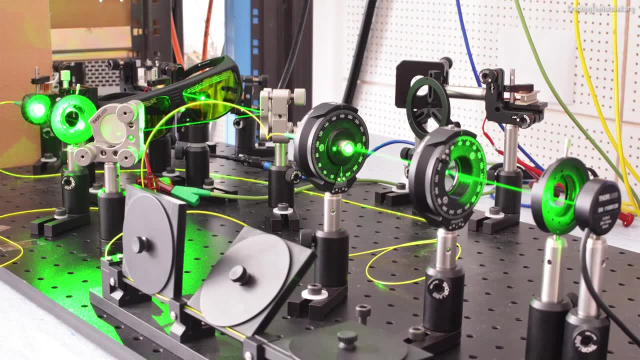 manifestation of certain pairs of these properties upon measurement. Complementarity is not something that manifests as a result of disturbances created by the properties of a particle at any given moment. In fact, it can be argued that, in reality, there is no actual physical wave and that there is no physical particle in the state of this. 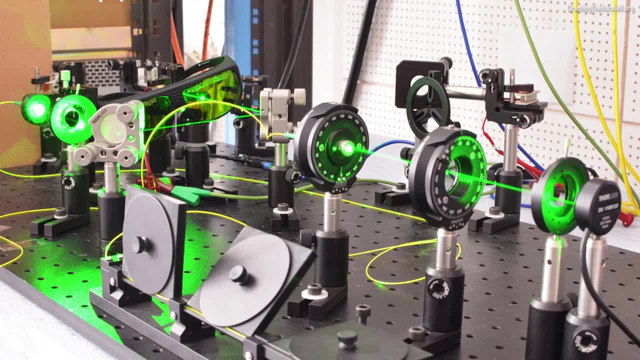 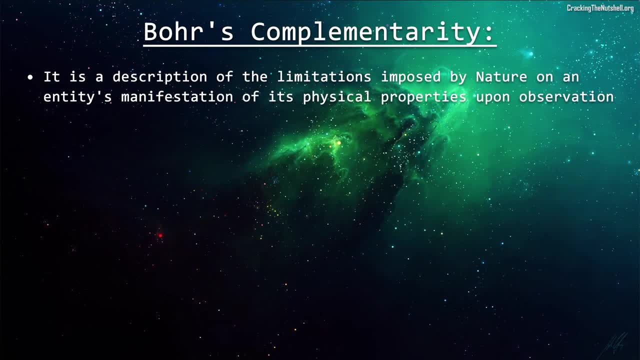 particle and that there is no physical particle in the state of a particle. Neither is it a result of instrumental limitations nor a reflection of our lack of knowledge. Complementarity is a description of the limitations imposed by nature itself on the physical entity's. 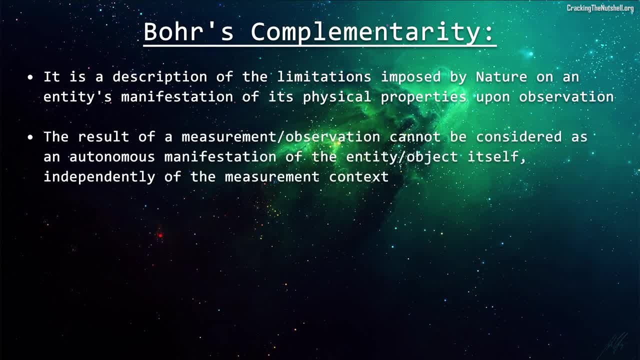 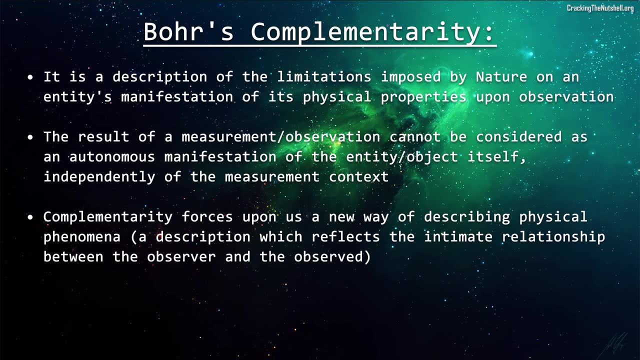 manifestation of its physical properties. The result of a measurement cannot be considered as an autonomous manifestation of the object itself, independently of the measurement context. Complementarity forces upon us a new way of describing physical properties, phenomena, a description which reflects the intimate relationship between the observer. 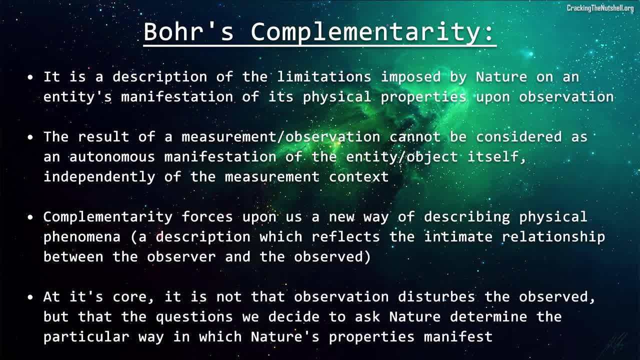 and the observed At its core. it's not that observation disturbs the observed, but that the questions we decide to ask nature determine the particular way in which nature's properties manifest. In other words, what we observe becomes manifest only in relationship to our 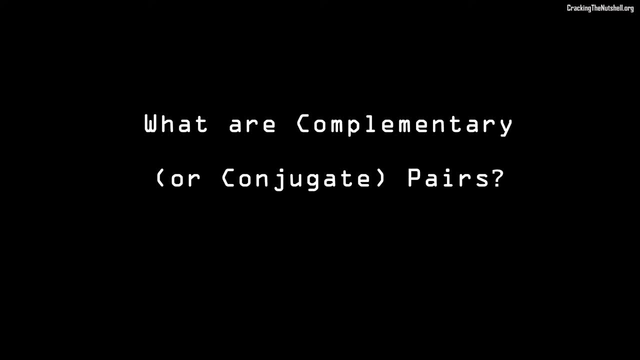 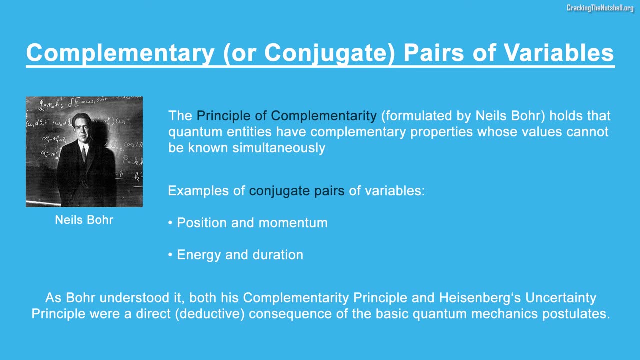 modes of questioning. At the heart of complementarity is the idea that all properties of physical entities exist in pairs and that, upon measurement, what we physically observe is defined by the manifestation of such properties, properties which are limited by trade-offs between these complementary. 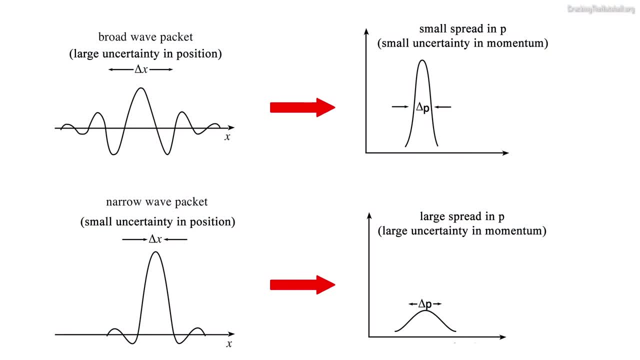 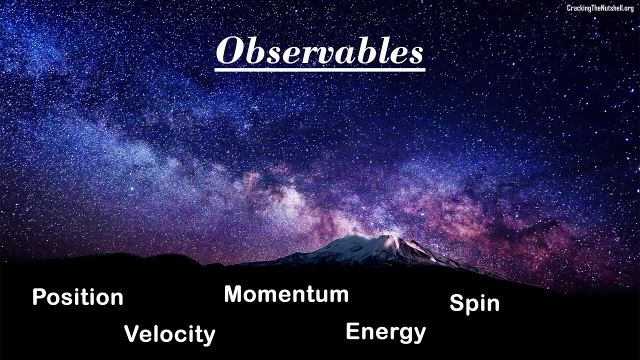 pairs. For instance, as we have seen, the greater accuracy in an electron's position is manifested only in a fair trade for the properties of physical entities. Therefore, a complementary loss of accuracy in the values of its momentum, Position, velocity, momentum energy, spin, duration are all examples of properties. they 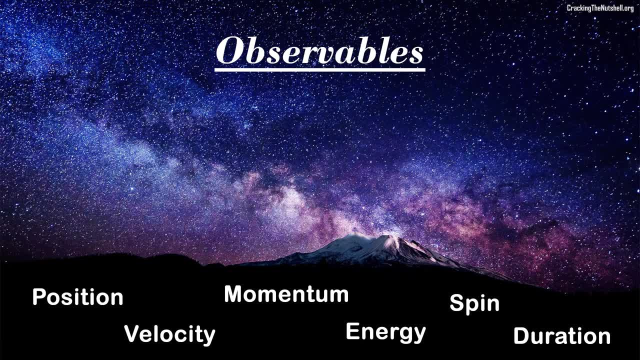 are what physicists call observables. They are observables because we can measure them, we can observe them, that is, we can bring about these properties from a realm of possibility to a realm of physicality. Well, turns out, these observables exist in pairs, and some 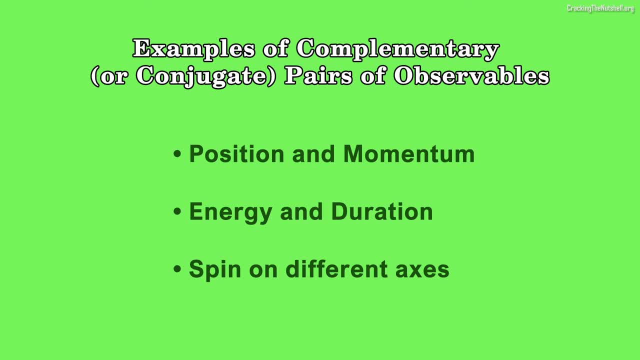 of these pairs, called complementary or conjugate. observables such as position and momentum, not only are indeterminate until measured, but they are also under nature's limitation that their precise values cannot be brought about simultaneously. In other words, as a result of this limitation imposed by nature as to how certain pairs of observables can 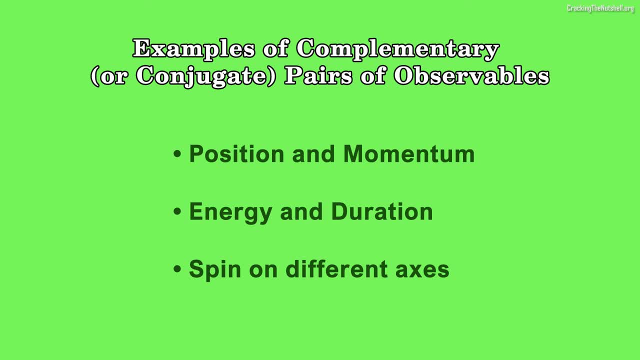 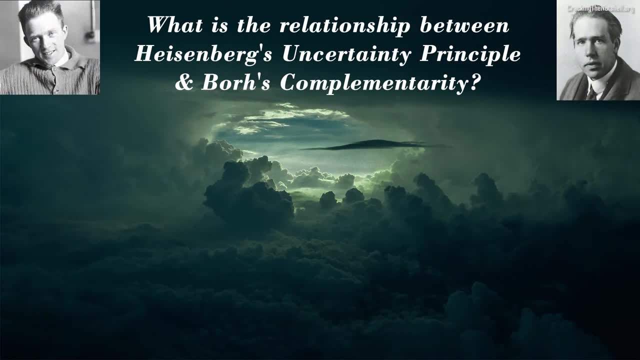 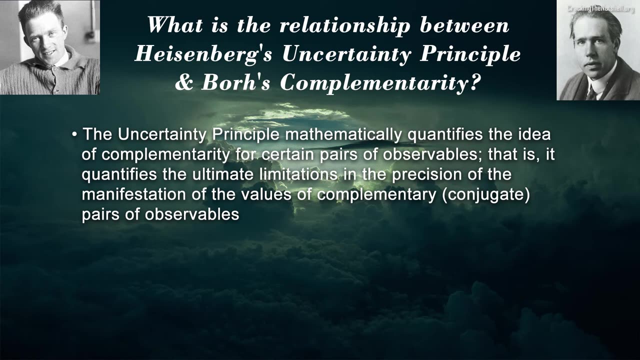 physically manifest, we cannot know the precise values of certain pairs of observables at the same time. So where does Heisenberg's theory come from? Well, what the uncertainty principle does is to mathematically quantify the ultimate limitations in the precision of the manifestation of certain complementary observables. As Bohr 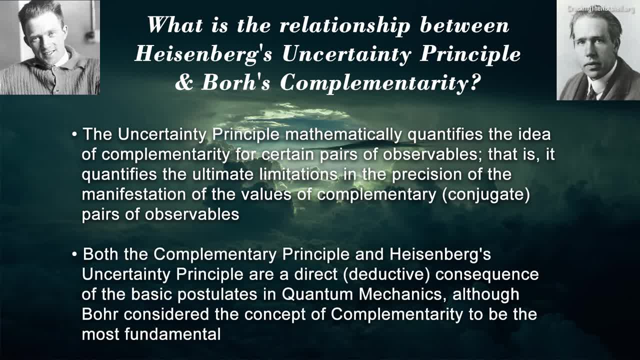 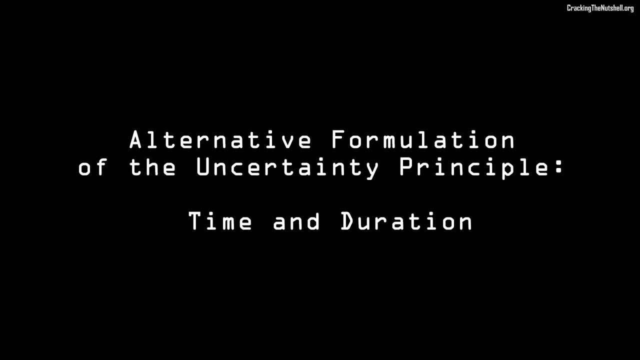 understood it. both his complementary principle and Heisenberg's uncertainty principle are a direct deductive consequence of the basic quantum mechanics postulates, although he considered the concept of complementarity to be the most fundamental. I'd like to end this video by showing you another important form of Heisenberg's uncertainty. 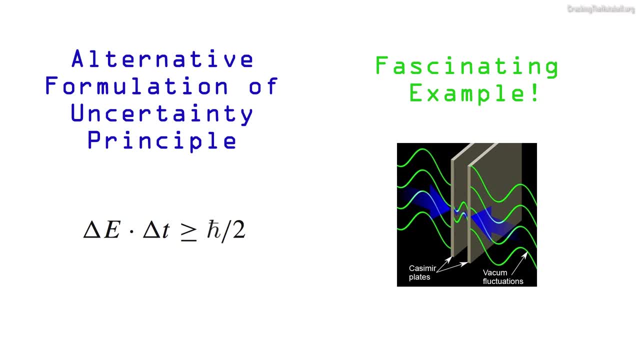 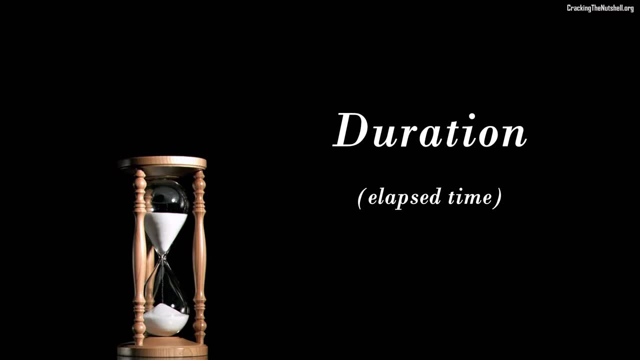 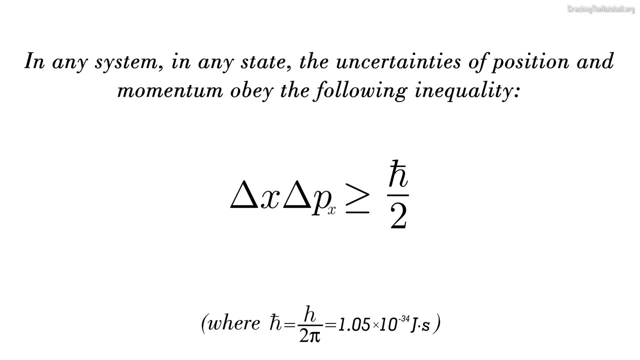 principle, followed by a very interesting example. Here's the conjugate pair we'll be dealing with this time – energy and duration. In my previous videos we saw what the uncertainty principle looks like for position and momentum. Here's a reminder. Well, for energy and duration, the uncertainty relationship takes two parts. The first part. is the energy and the duration. The second part is the momentum. The third part is the energy and the duration. The third part is the momentum. The fourth part is the momentum. And now let's look at theochromatic number, an analogous form: Here in this unit you 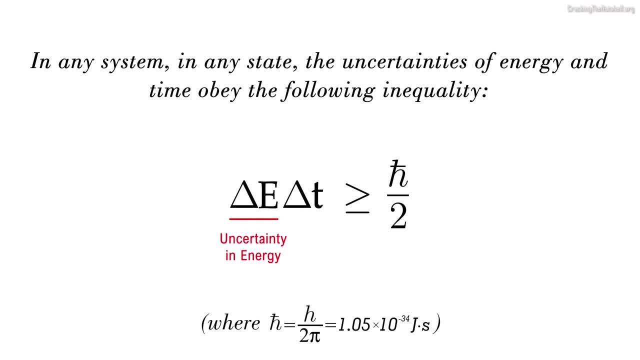 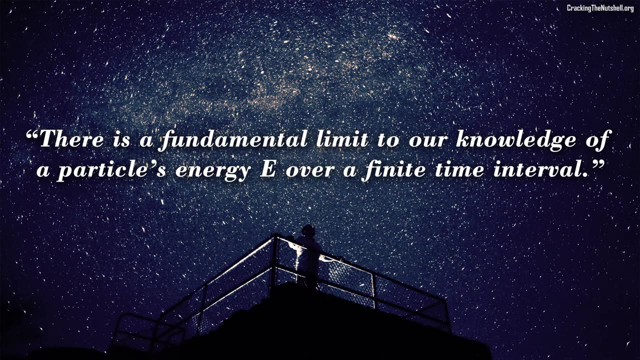 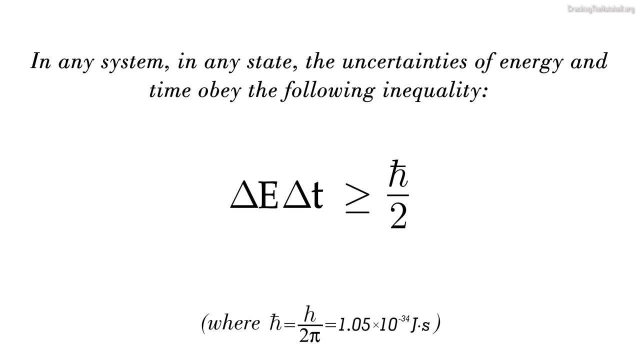 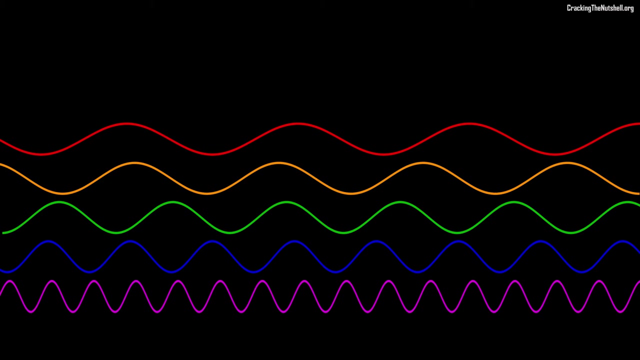 can find it each time in�sose time blank, a finite time interval. What this formula does is to quantify the limitations to the precision with which the energy of the particle can be known. As you saw in my previous video, where I covered the case of position and momentum, it is possible to see intuitively how these limitations arise. 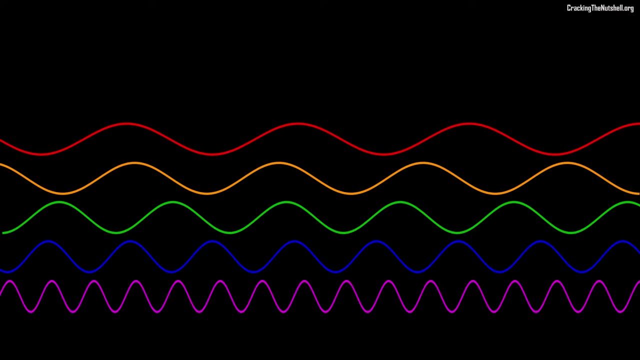 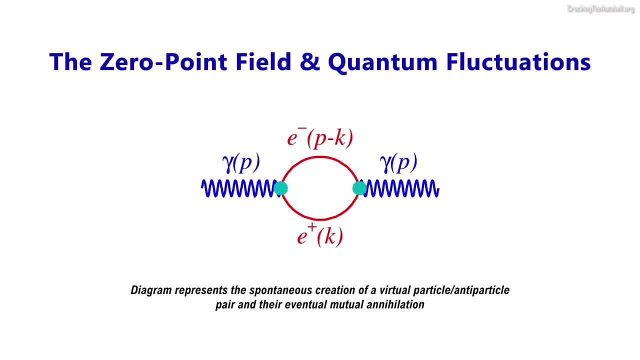 as soon as matter or light are described in terms of probability waves. Well, the same underlying ideas apply for energy and duration. Here is a very interesting example which can actually be explained by applying the uncertainty principle to energy and duration. Let's start with virtual particles. A virtual particle. 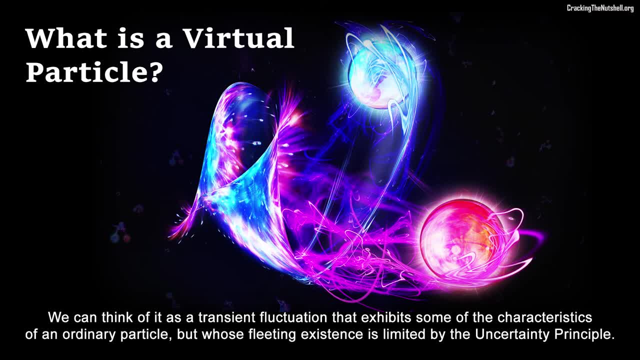 can be defined as a transient fluctuation that exhibits some of the characteristics of an ordinary particle, but whose fleeting existence is limited by the uncertainty principle. But how is that so? The energy of the particle is limited by the uncertainty principle, but the energy of the 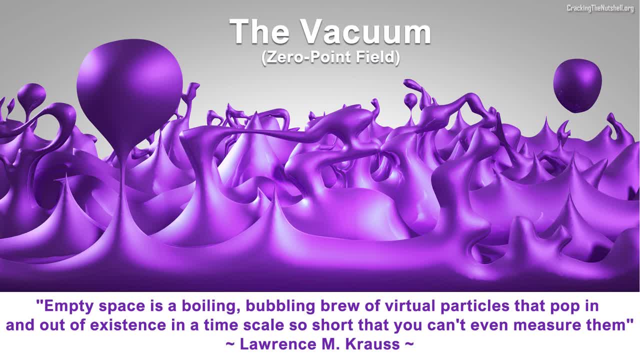 vacuum can fluctuate in such a way that unobservable virtual particles can pop in and out of existence all the time. Thanks to the uncertainty principle, what we call empty space is actually a boiling bubbling brew of virtual particles that pop in and out of existence in a time scale so 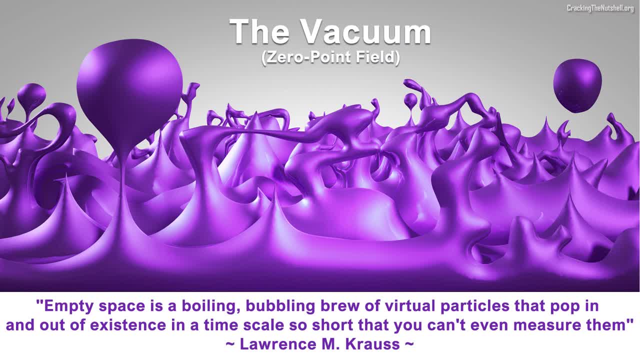 short, that it is impossible for us to measure them. The existence of such particles is possible because at every point in spacetime, even in a perfect vacuum, the vacuum is constantly changing, And that is possible. through a perfect vacuum, there is always an uncertainty in energy and an uncertainty in duration. 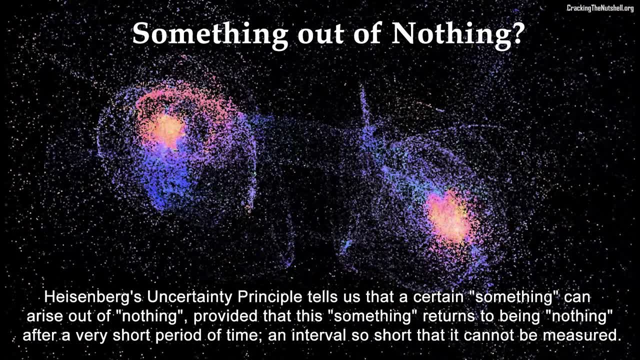 Here's a more poetic way of describing this fascinating phenomenon. Heisenberg's uncertainty principle tells us that a certain something can arise out of nothing, provided that this something returns to being nothing after a very short period of time, an interval so short that it cannot be. 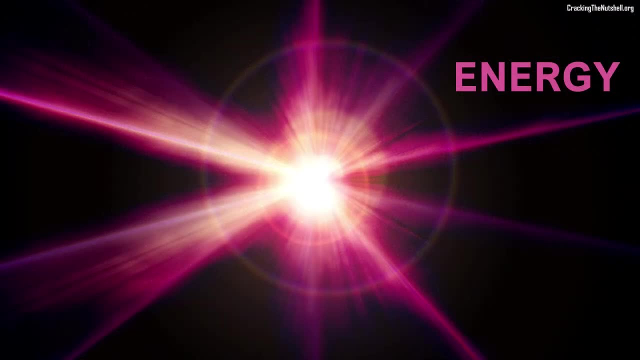 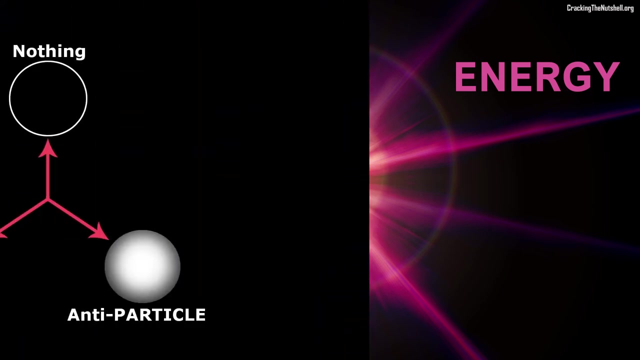 measured. I find it fascinating to think that the creation of these virtual particles can also be thought of as a kind of micro-violation of the law of conservation of energy. I mean, these particles pop in and out of existence all the time thanks to the uncertainty principle, And so empty space. 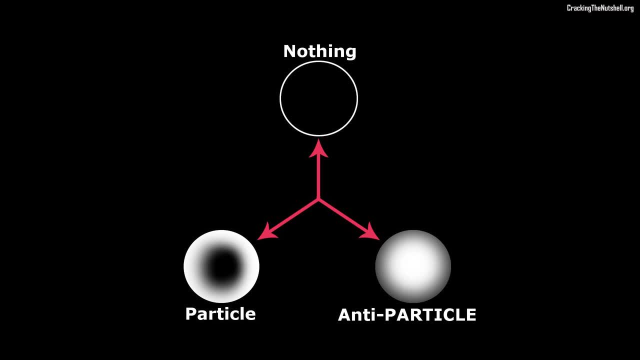 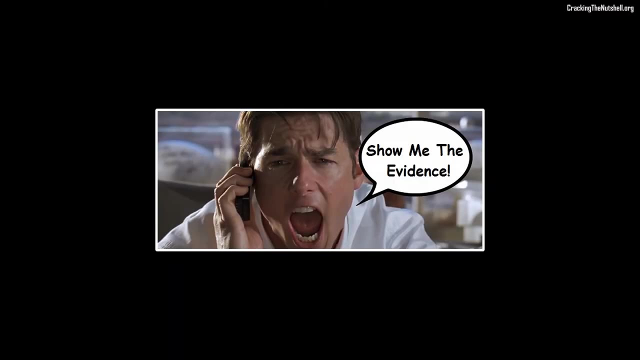 is seeding with particle-antiparticle pairs that come into being and then annihilate each other, And this happens over and over again, their existence being confined to a failure to be realized, A fleeting, minuscule moment in time. But hold on a second. Where is the evidence for all this, you may wonder? Well, turns out that this: 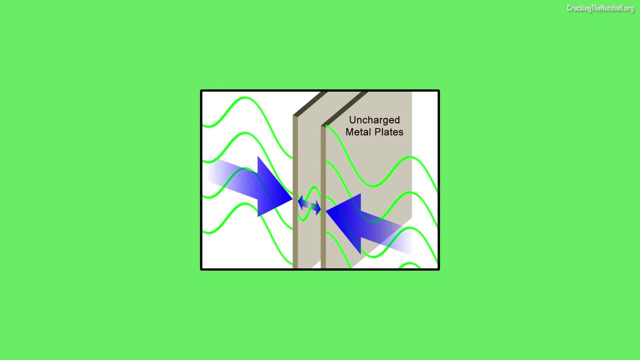 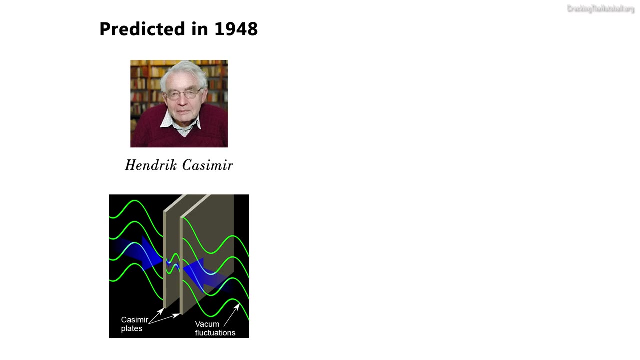 something-from-nothing phenomenon can actually be shown to work its magic between something as simple as two plain metal plates, Which brings me to the Casimir effect. In 1948, Dutch physicist Hendrik Casimir predicted that one consequence of the zero-point field is an attractive 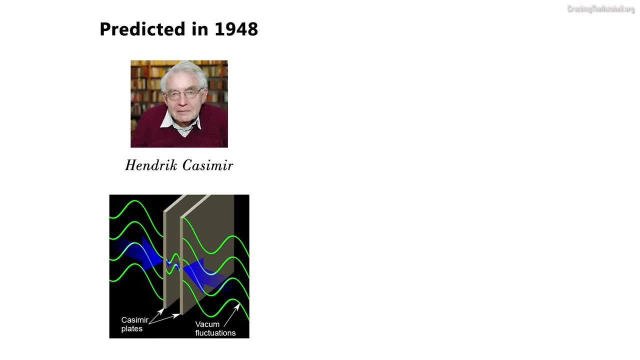 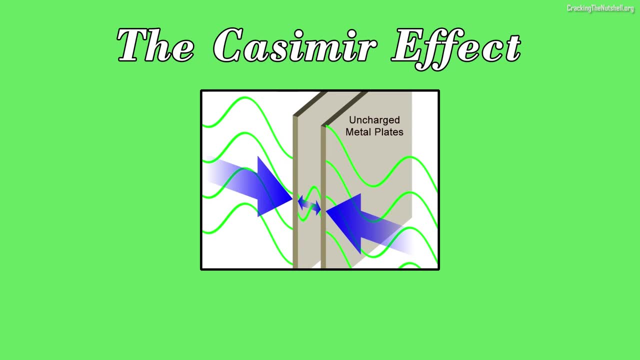 force between two uncharged, perfectly conducting parallel plates, a phenomenon which became known as the Casimir effect. The Casimir effect is a force which literally seems to emerge out of nowhere, a vacuum force which manages to push the two metal plates together, Even though Casimir predicted the 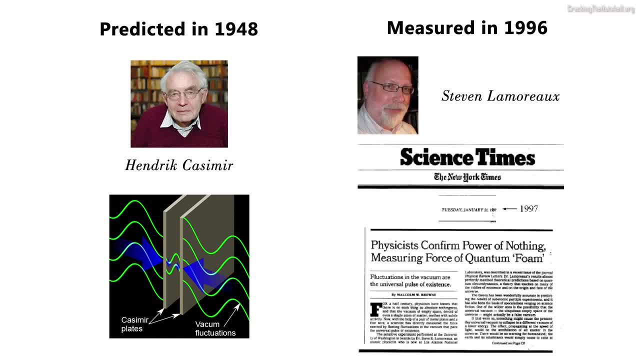 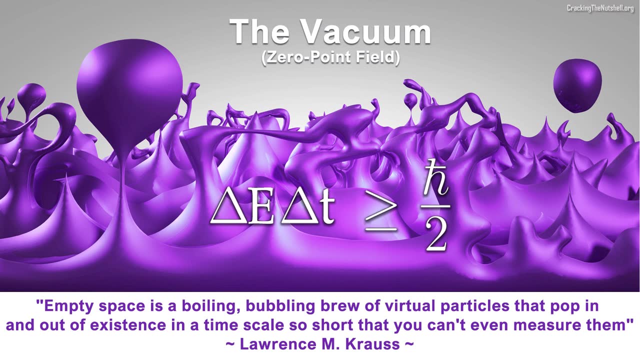 effect in 1948, it was actually not until 1996 that Steven Lamoureux, now at Los Alamos National Laboratory, measured the effect for the very first time. The Casimir effect takes place because, thanks to Heisenberg's uncertainty principle, the energy of the vacuum can never be zero at any particular moment in time. 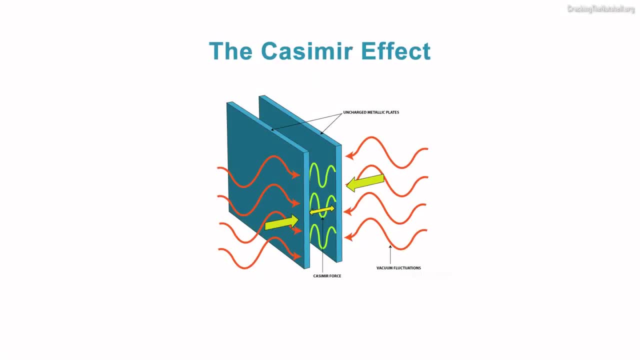 There is always uncertainty. This allows for the virtual particle pairs to be created, which in turn produce photons which apply a force to the plates from both inside and outside the gap. If we make the distance inside the gap small enough, photons with a larger wavelength than the gap between the plates can be created. 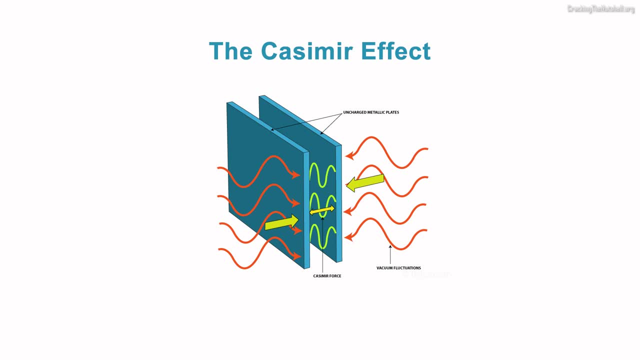 Hence, an imbalance of forces takes place between the outside and the inside of the plates. And so voila, Because the force pushing from the outside is larger than the force pushing from the inside, the metal plates end up moving towards each other. 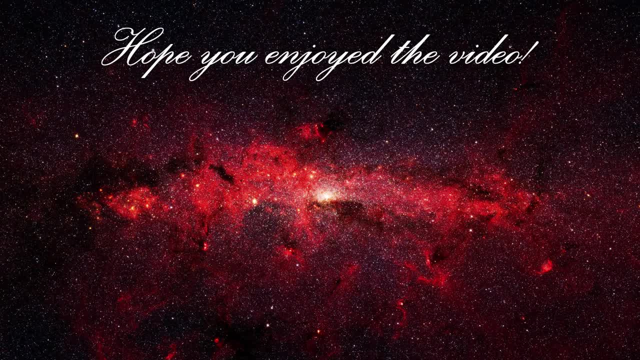 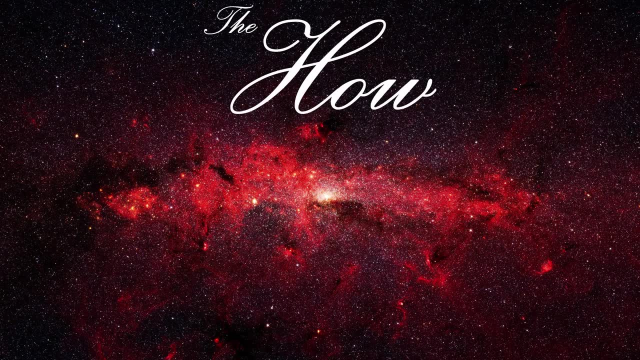 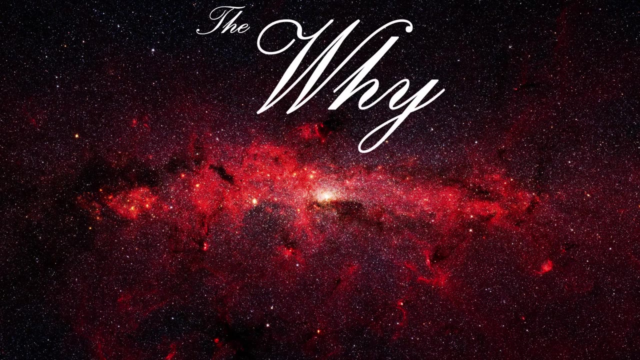 I hope you have enjoyed this third video in the series and that it gives you an even wider understanding of Heisenberg's uncertainty principle. So far we have answered the question of how Heisenberg's uncertainty principle arises, But perhaps the most intriguing question is why? Why are complementarity and indeterminacy? 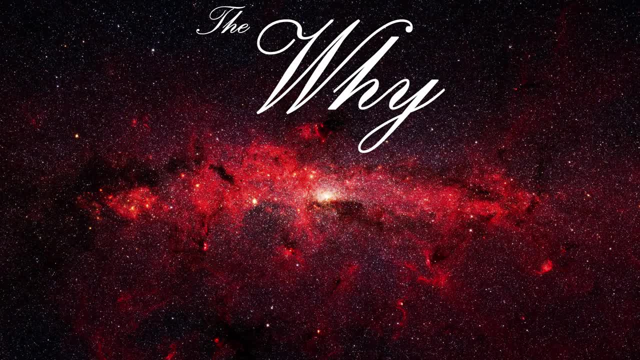 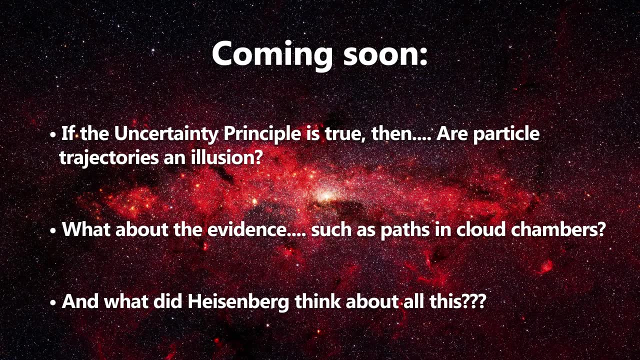 at the heart of quantum mechanics. This is the million-dollar question which I'll attempt to cover very soon in this series, But before that, in my next video, I'll talk about particles, trajectories and cloud chambers and how all of these relate to Heisenberg's uncertainty. 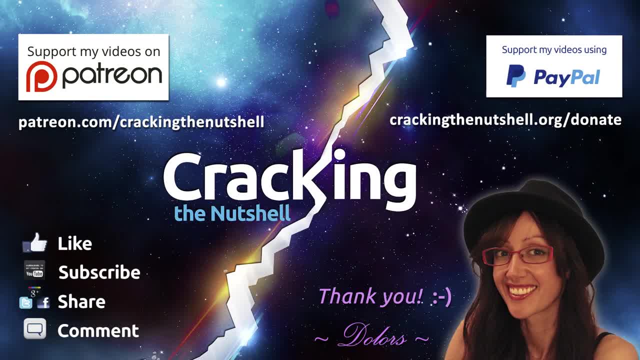 principle. Thank you for watching and thank you so much for your support. I would not be here without it. Stay tuned and see you very soon.